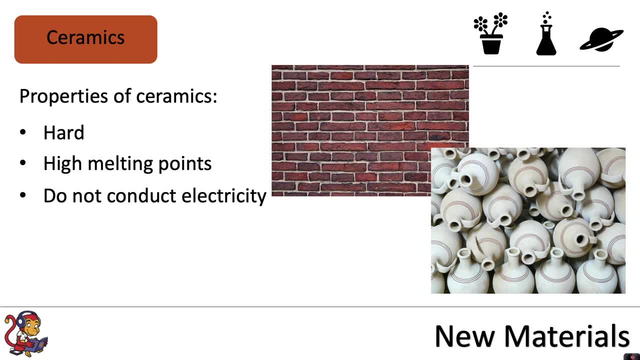 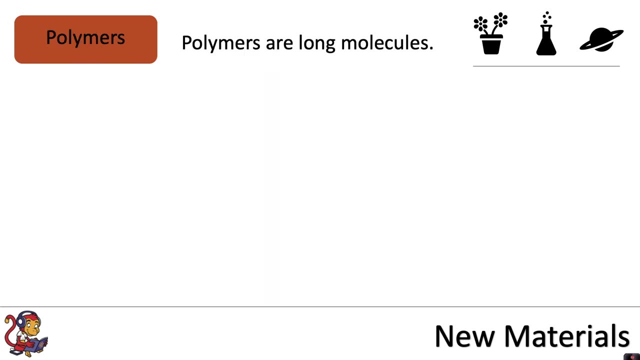 They don't conduct electricity. but perhaps one property that isn't so useful is the fact that they are brittle. So if you were to hammer the pottery or the bricks they would shatter and break up. Polymers are long molecules. Polymers are made in chemical reactions that join lots. 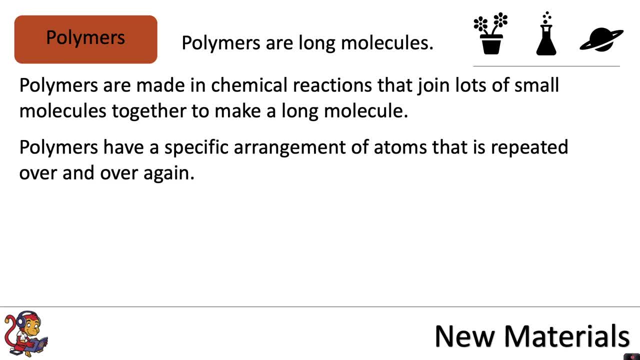 of small molecules together to make a long molecule. Polymers have a specific arrangement of atoms that is repeated over and over again. For example, if we started off with a small unit of atoms to make a polymer, we'd have to join lots of those up in one long chain of repeated units. 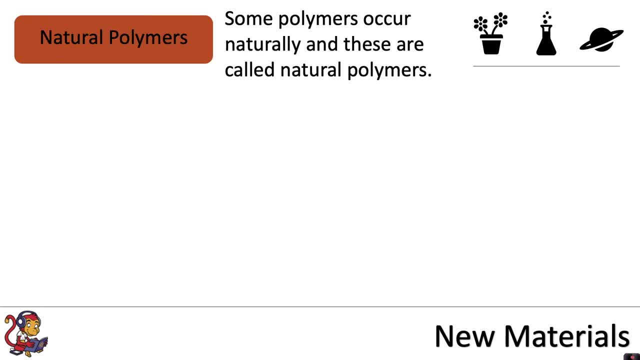 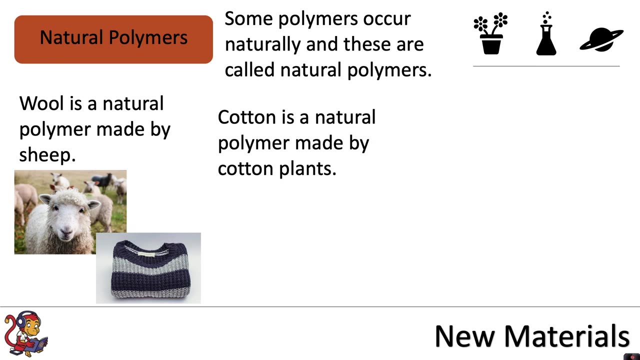 Some polymers occur naturally, and these are called natural polymers. wool is a natural polymer made by sheep, and wool is a really useful material used in clothing. cotton is a natural polymer made by cotton plants and again, we use this mainly in clothing. 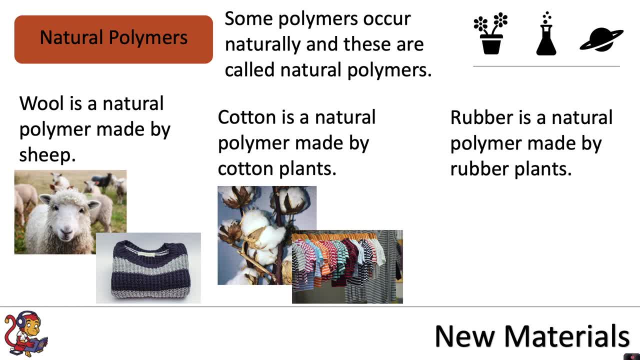 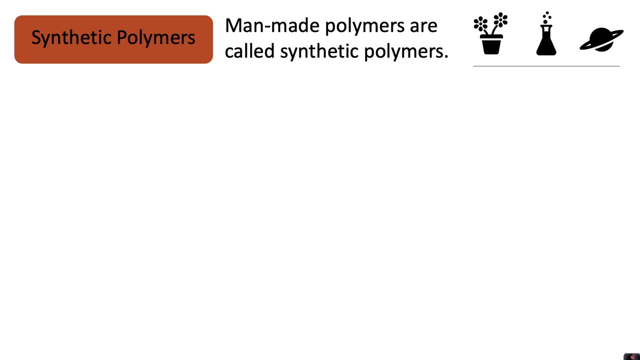 and rubber is a natural polymer made by rubber plants, and this can be used to make things such as tires, although nowadays, rubber tires are normally made out of man-made rubber. man-made polymers are called synthetic polymers. plastics are synthetic polymers to make plastic. crude oil is extracted from deep under the sea. 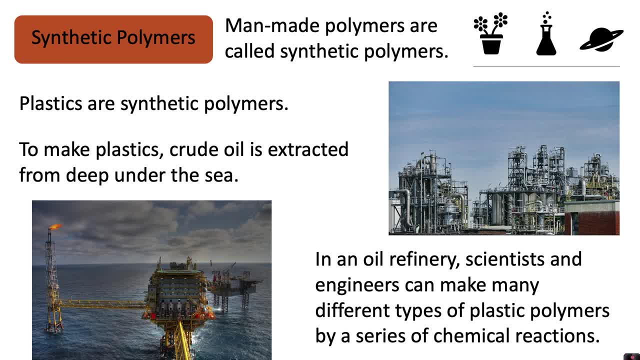 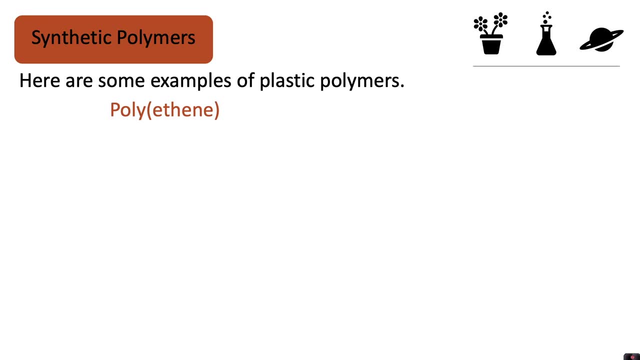 in an oil refinery. scientists and engineers can make many different types of polymers, and they can be used to make different types of plastic polymers by a series of chemical reactions. here are some examples of plastic polymers. polyethene, or otherwise known as polythene, is an example of a plastic polymer, and there are two. 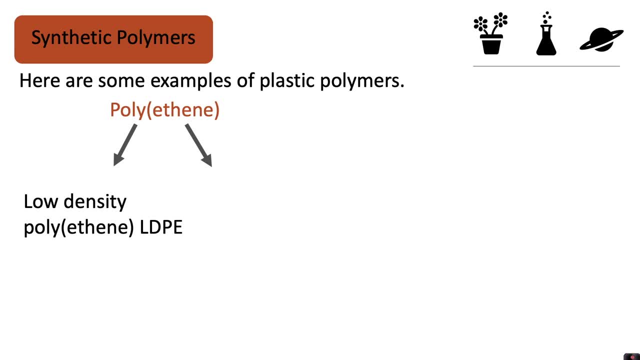 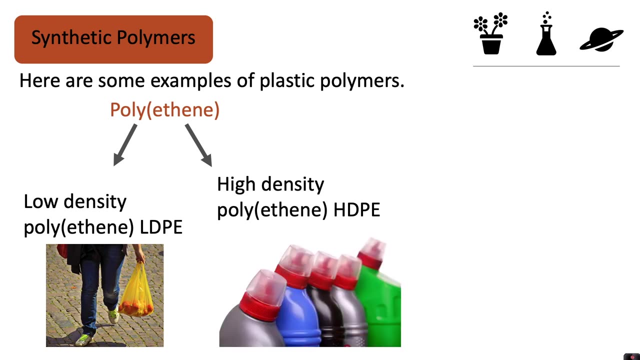 types. low density polyethene, or ldpe, is used to make things such as plastic bags, and high density polyethene, hdpe, is used to make harder plastics such as bottles and pipes. another example of a plastic polymer which is man-made is poly vinyl chloride, otherwise known. 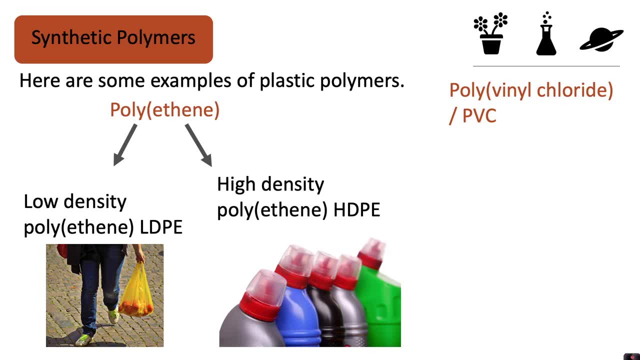 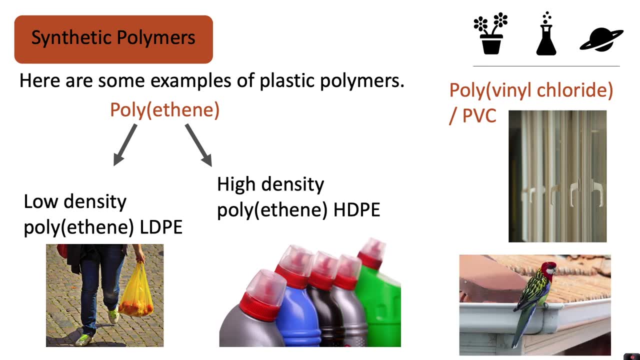 as pvc and that is used to make things such as window frames and guttering. properties of polymers include the fact that they are strong, so that's really, really useful, and they're made of high density polyethene. that's why it's called a polythene polymer. 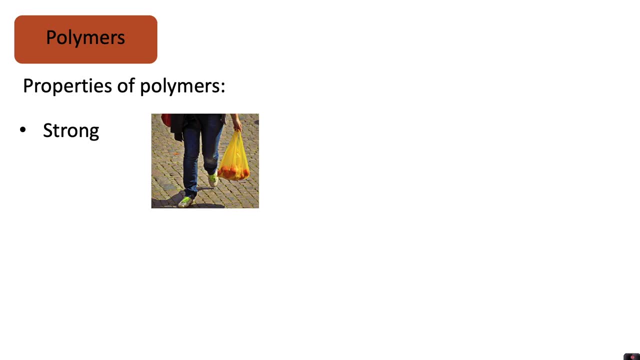 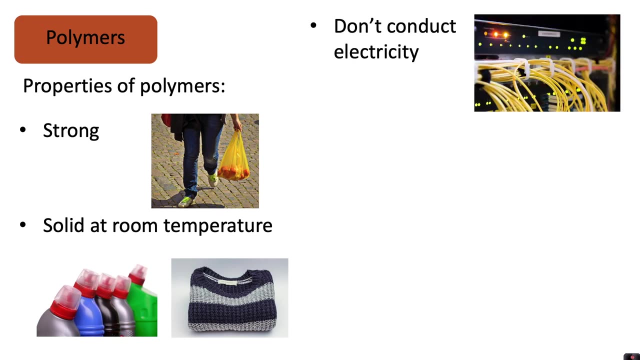 useful in case of a plastic bag when you're wanting to carry things. They are solid at room temperature. They don't conduct electricity, so that's why our wires are coated in a plastic polymer, because then we can hold the wires without getting an electric shock. They are unreactive, which is really useful. 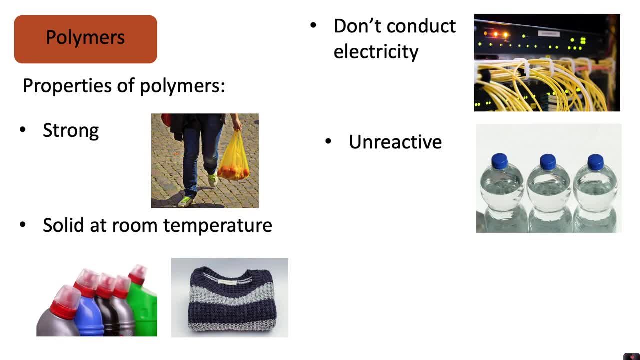 because they can be used to store things such as food and water, but there is a problem with the fact that they're unreactive, and the problem is when they are placed into landfill, because when they are placed into landfill, they will remain there for thousands of years because they do not naturally biodegrade. 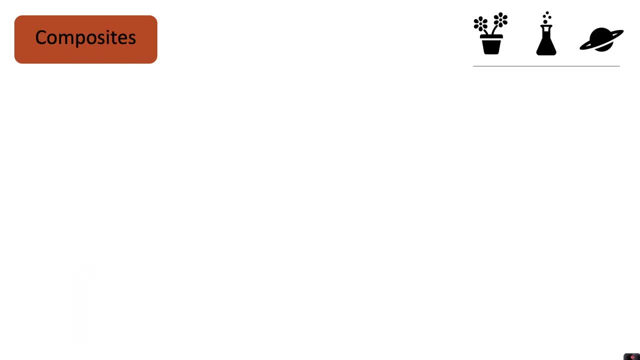 Our third material that we're going to look at is the composite. The composite is a mixture of materials. Two or more materials are combined to make a material which has the favourable properties. So if you like the properties of one type of material and you like the 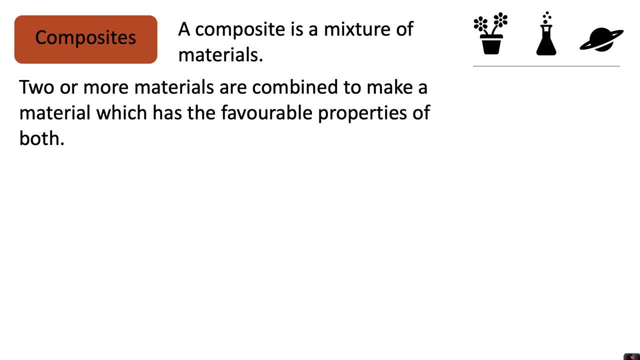 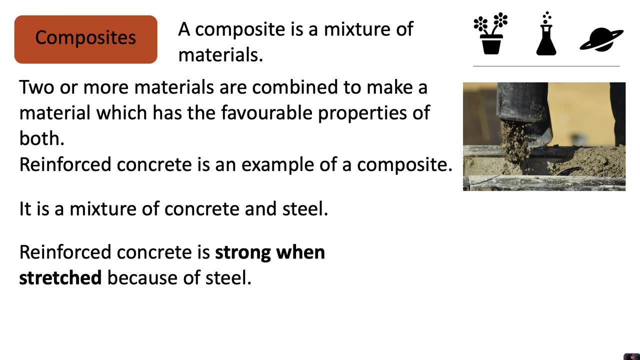 properties of another type of material. you might want to combine those together to make a composite. Reinforced concrete is an example of a composite. It is a mixture of concrete and steel. Reinforced concrete is strong when it's stretched because of the steel and it is strong when it's stretched because of the steel. 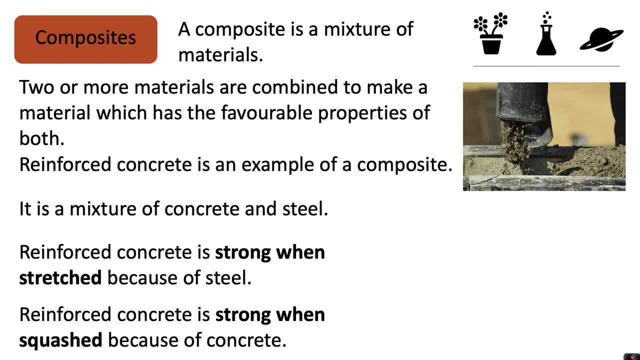 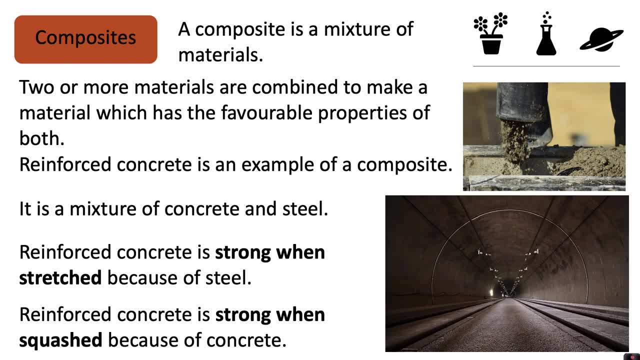 It is strong when squashed because of the concrete, So the mixture of these properties makes it an extremely strong material that is used for building, so building tunnels and bridges and buildings, etc. This new composite material has proven to be an excellent material because the mixture of